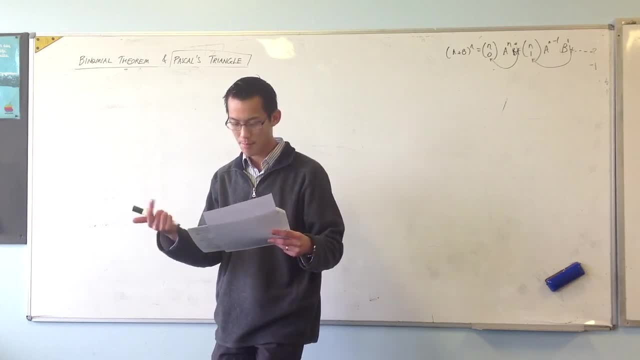 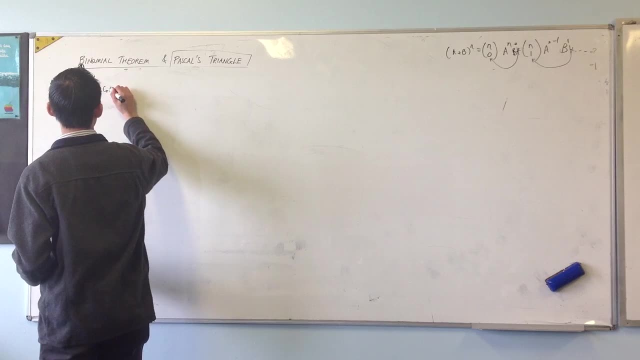 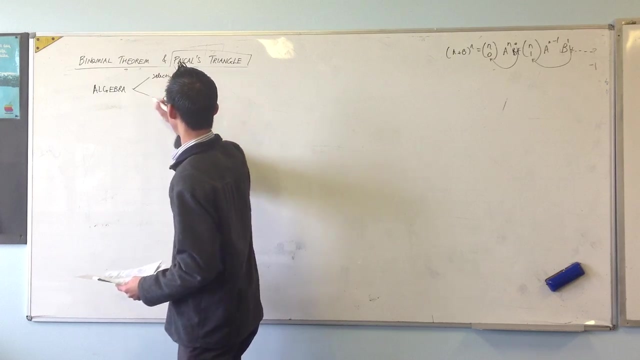 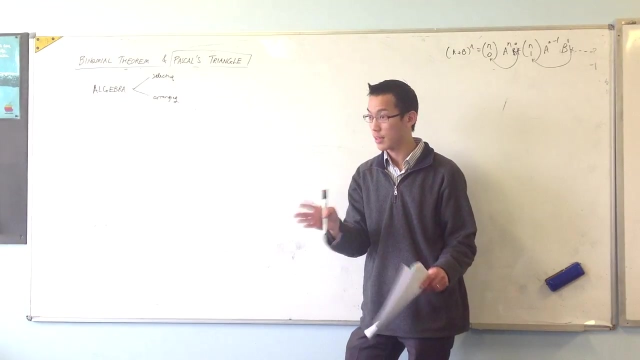 How many ways are there of selecting, arranging three letters of the word Algebra? So the first one is selecting and then the second one is arranging. So obviously one order matters and one the order doesn't. The way we were thinking about it before is: look, there are seven letters and you want three. 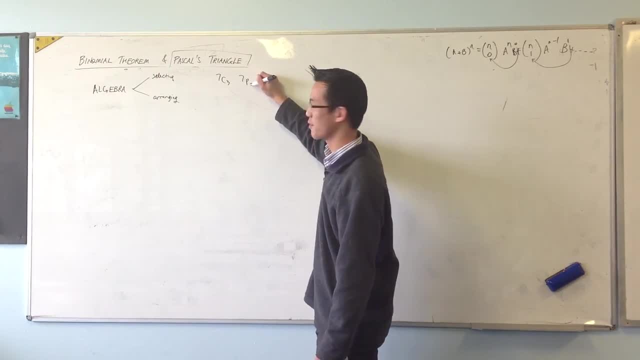 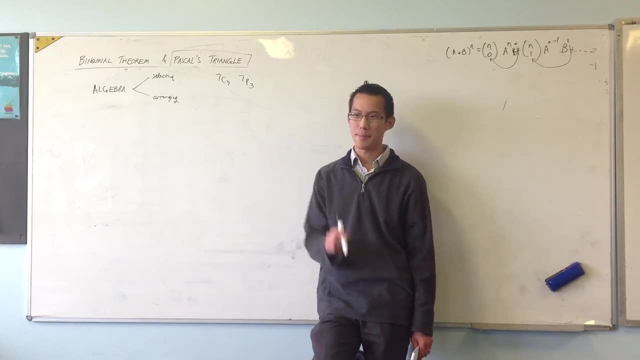 so it's got to have something to do with seven choose three, or seven pick three, or something like that. Except, you don't get the right answers. and the question is why- And that's why I always hated about perms and comms, because it's like: what am I missing? 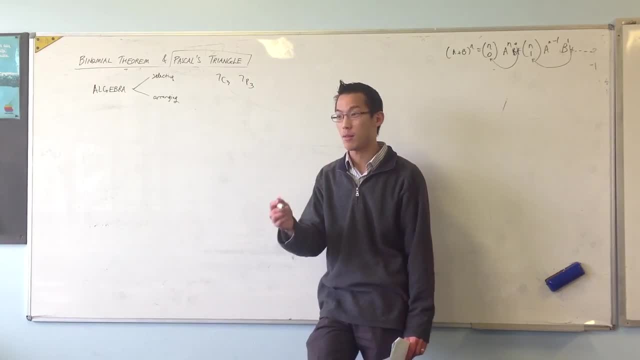 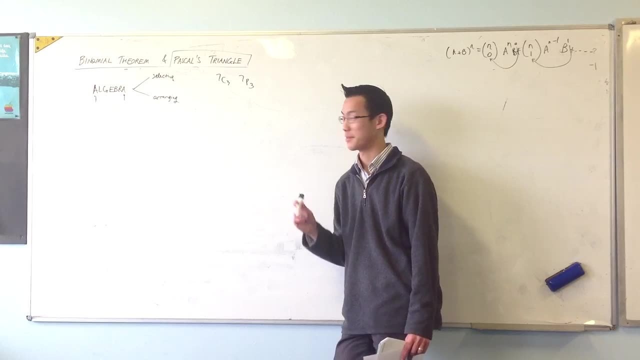 Looks fine to me, isn't it? You can notice that one of the problems will be: you've got these two A's, So that repetition causes you issues. That's what makes this a tricky question, But simply dividing by two turns out to be not a very useful approach. 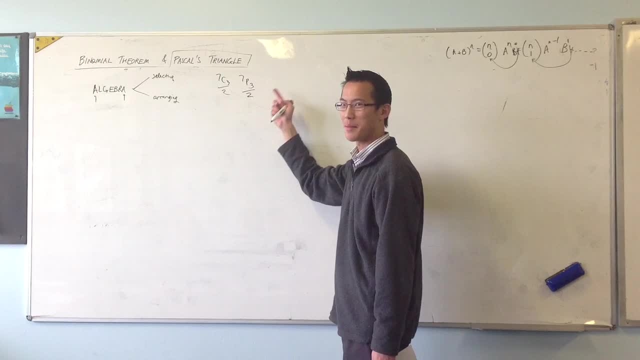 because I think, which one is it? One of these is an odd number, So you divide by two and you get a half of a way. So it's like it's kind of a way, but it's not a very good one. 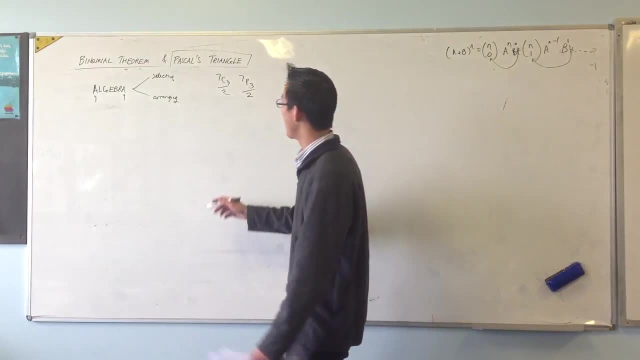 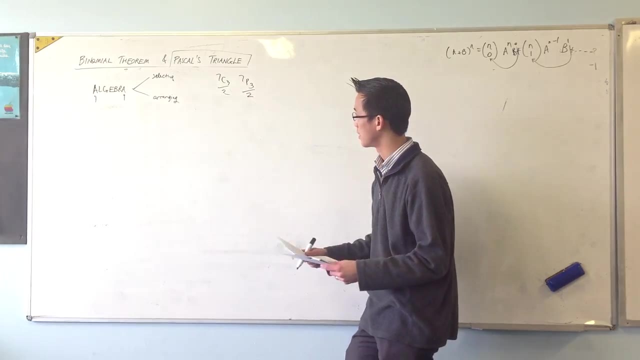 What does that even mean? So here's the way that I would go about it. Now, let me make sure I do it in the right order When you're selecting, so I don't care about which order I get them in. you've got to be careful with these A's. 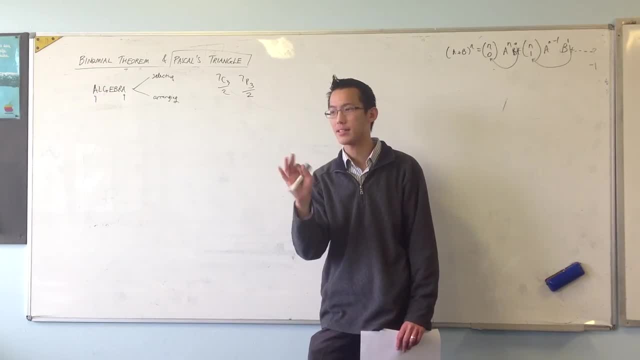 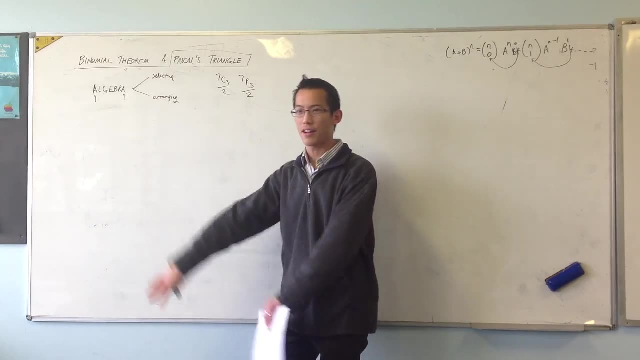 So here's the way that I would think about it. There are three basic ways you can make a three-letter word, And what I'm going to do is, because the A's are the problem, I'm going to take them out of the equation as a variable. 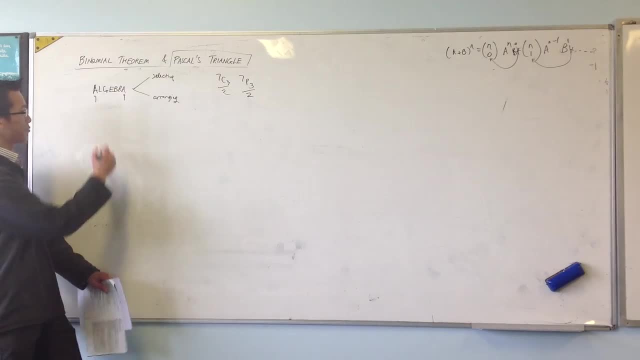 So I'm going to think about the three ways, as here's one way, Method number one: I could have no A's, So just forget about the fact that there are A's for a second. That means I've got five different letters to choose from. 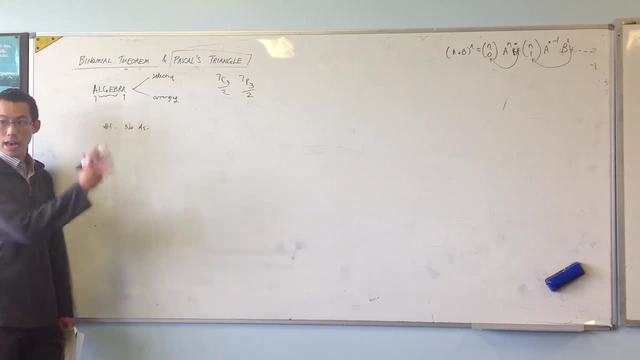 L, G, B, R. So how many ways are there to make a three-letter word when I've got no A's to choose from? Answer: Remember, I'm not caring about order. So is it C or P? It's C, That's exactly right. 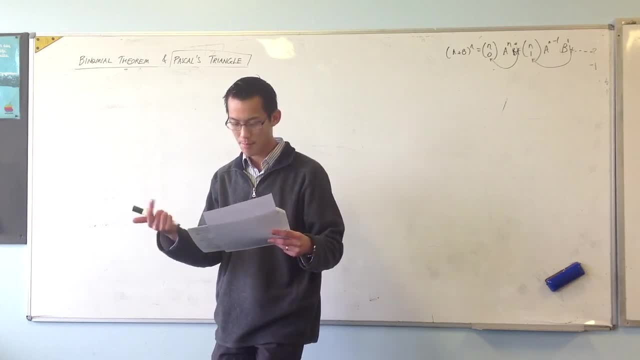 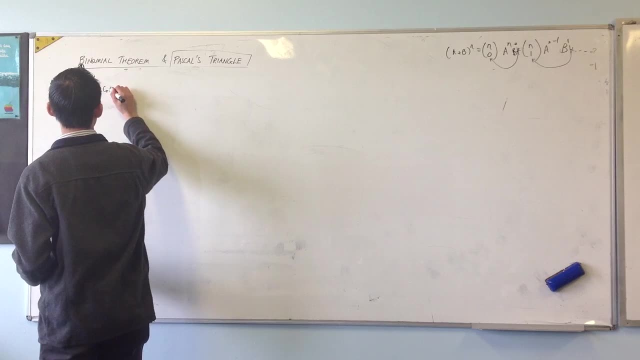 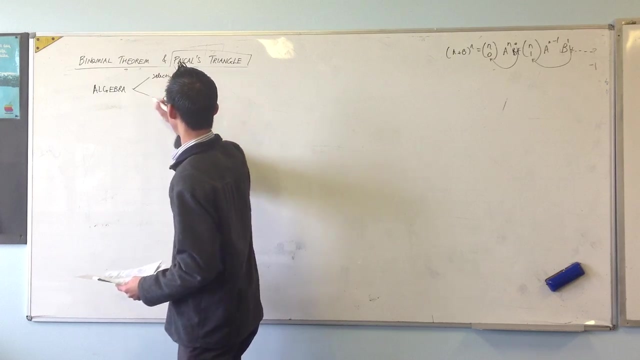 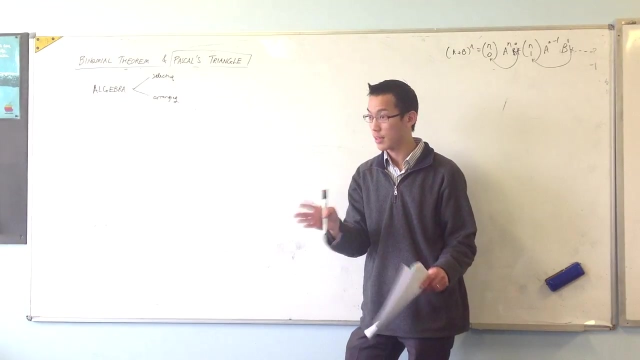 How many ways are there of selecting, arranging three letters of the word Algebra? So the first one is selecting and then the second one is arranging. So obviously one order matters and one the order doesn't. The way we were thinking about it before is: look, there are seven letters and you want three. 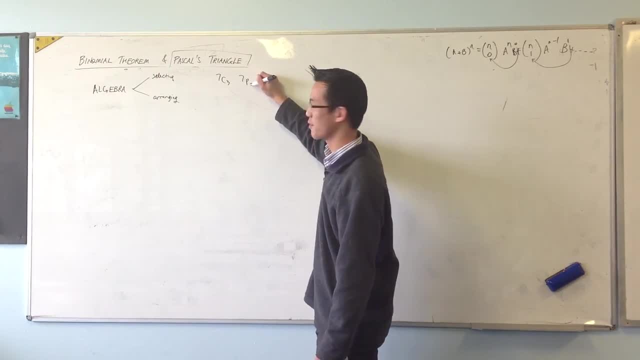 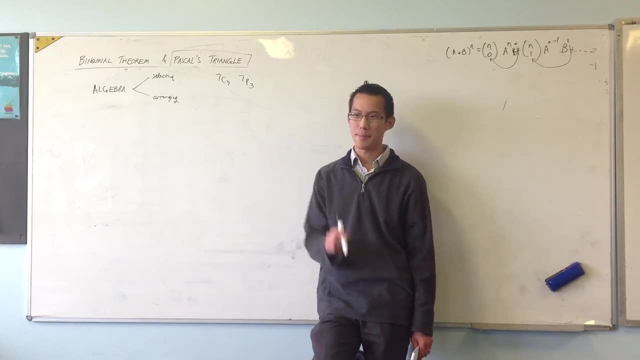 so it's got to have something to do with seven choose three, or seven pick three, or something like that. Except, you don't get the right answers. and the question is why- And that's why I always hated about perms and comms, because it's like: what am I missing? 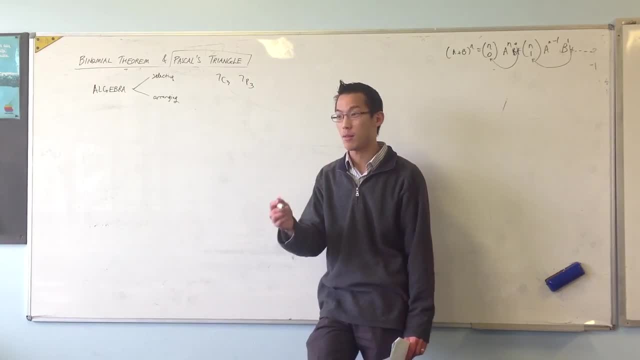 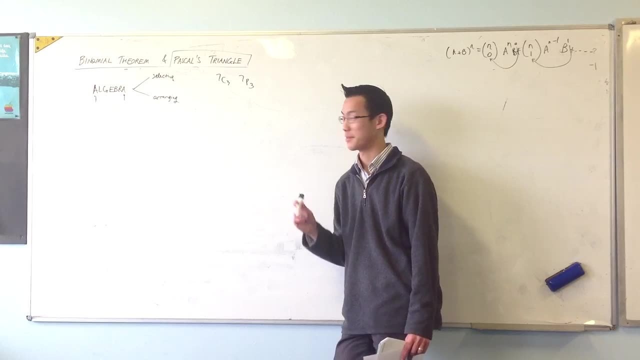 Looks fine to me, isn't it? You can notice that one of the problems will be: you've got these two A's, So that repetition causes you issues. That's what makes this a tricky question, But simply dividing by two turns out to be not a very useful approach. 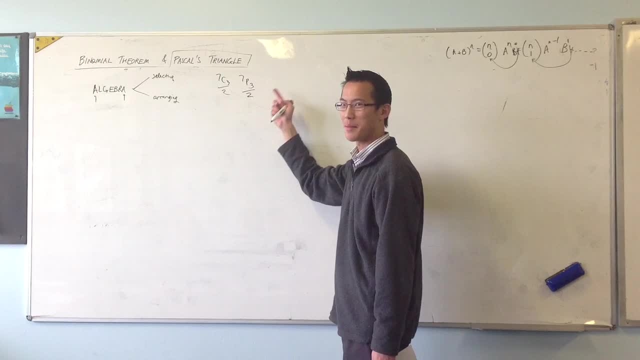 because I think, which one is it? One of these is an odd number, So you divide by two and you get a half of a way. So it's like it's kind of a way, but it's not a very good one. 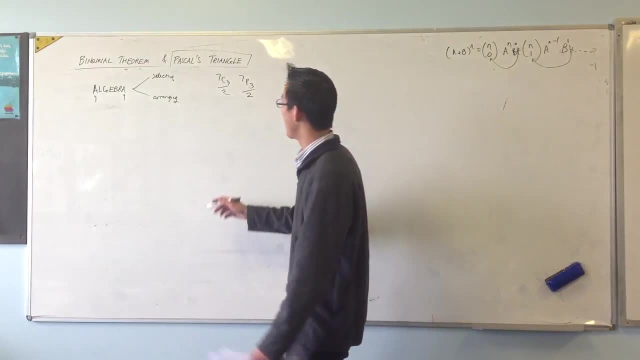 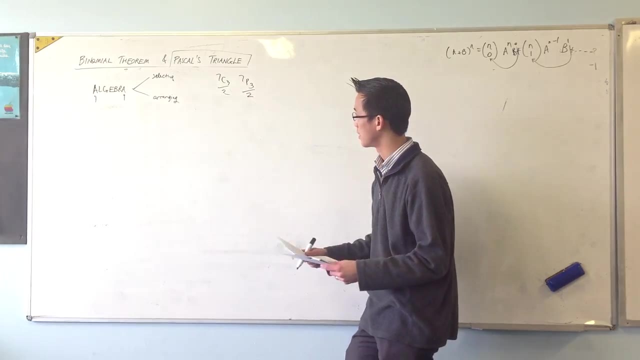 What does that even mean? So here's the way that I would go about it. Now, let me make sure I do it in the right order When you're selecting, so I don't care about which order I get them in. you've got to be careful with these A's. 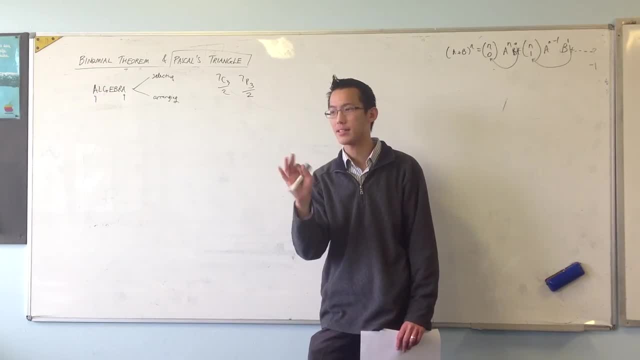 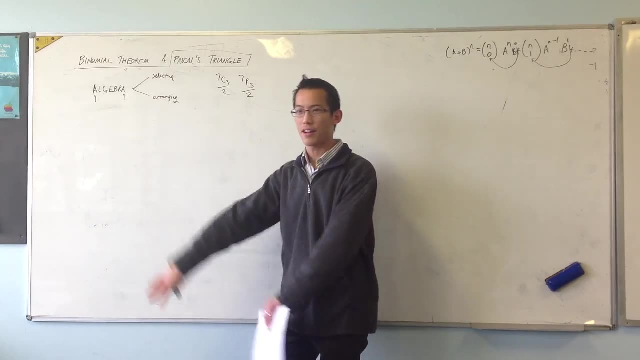 So here's the way that I would think about it. There are three basic ways you can make a three-letter word, And what I'm going to do is, because the A's are the problem, I'm going to take them out of the equation as a variable. 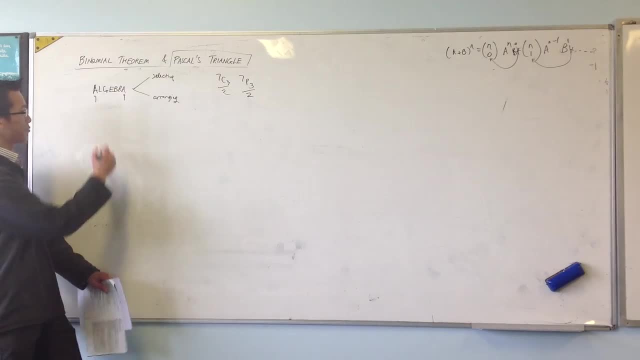 So I'm going to think about the three ways, as here's one way, Method number one: I could have no A's, So just forget about the fact that there are A's for a second. That means I've got five different letters to choose from. 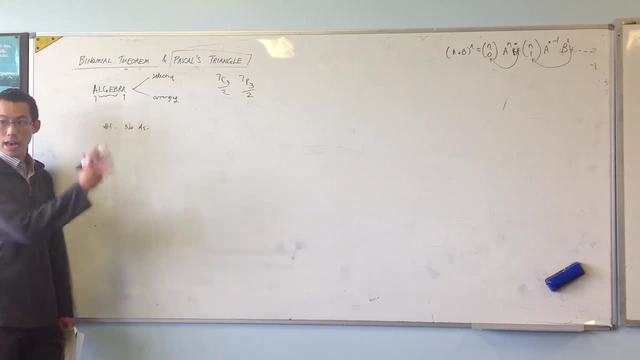 L, G, B, R. So how many ways are there to make a three-letter word when I've got no A's to choose from? Answer: Remember, I'm not caring about order. So is it C or P? It's C, That's exactly right. 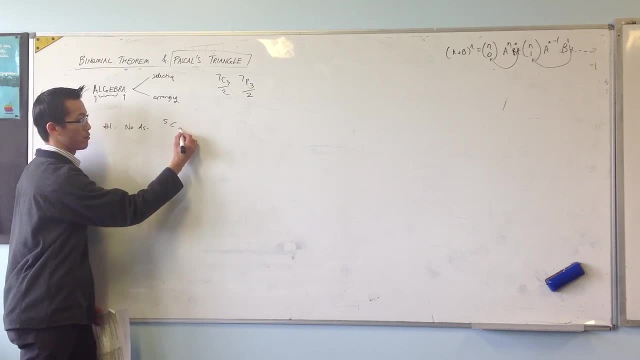 If I don't care about order. I've got five to choose from and I've got to choose three of them. Is that all right? Now, the second way is what if I have just one A? Now, don't forget, I don't care where the A is. 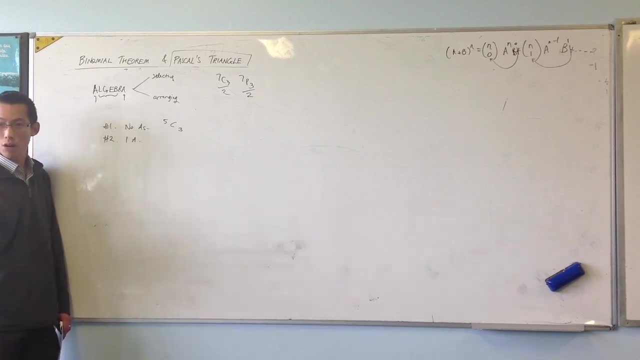 It could be at the start or the middle. at the end, If I've already chosen the A, I've got to make the other two letters from one of these five, And again I don't care what order. So I still have five to choose from, but I'm not choosing three. 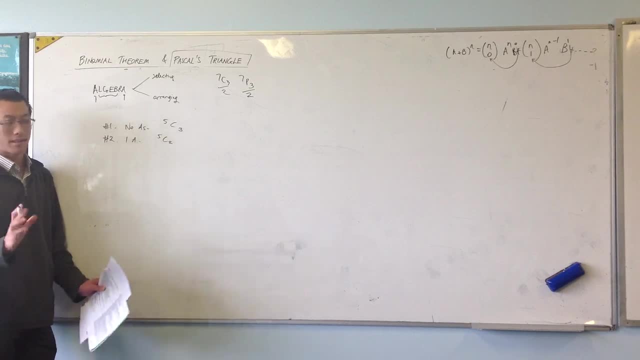 I'm choosing two. Last way. the third method is: what if I use both A's, So I could have them at the end, or I could have them bunched on the start or bunched at the end, But whichever way, remembering that I don't care about order, 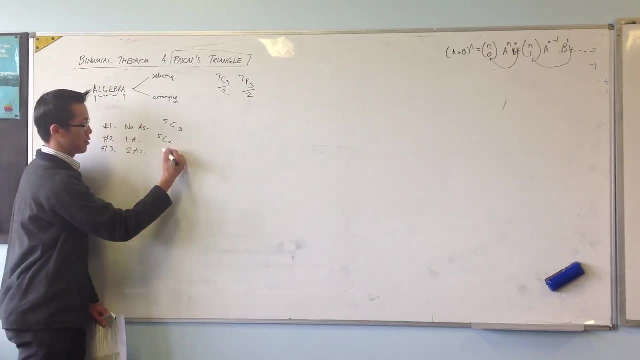 I have to pick one more letter to fill it out and I have to choose from five. So it's five, choose one. So when you add all of them up, I think you get 25.. This would be five, This is ten, and this is ten as well. 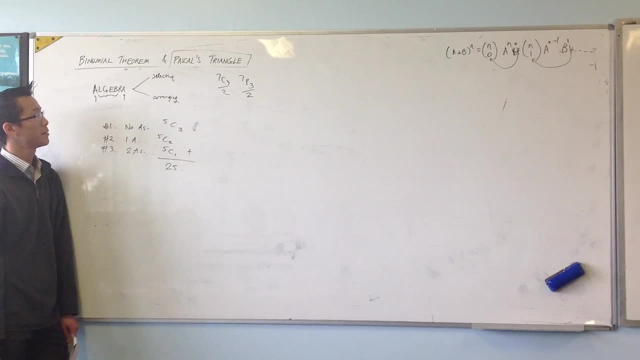 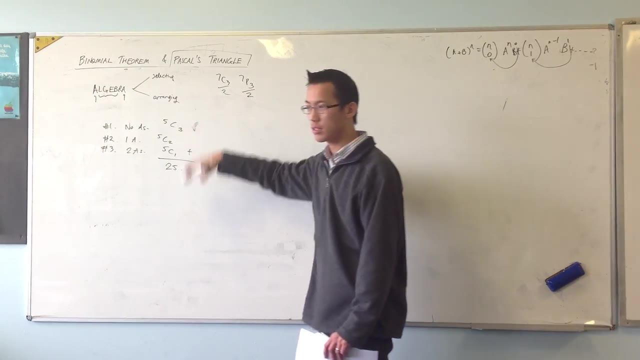 I think that's the way it works. So there's your 25,, which is the answer. How, then, do you go about it when you think about when order matters? You've still got to do a similar thing here. Let me make sure I read this properly. 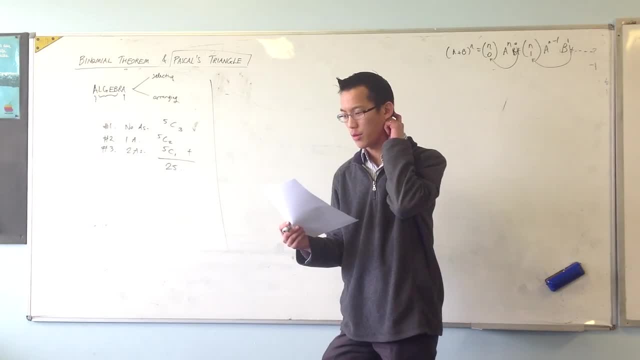 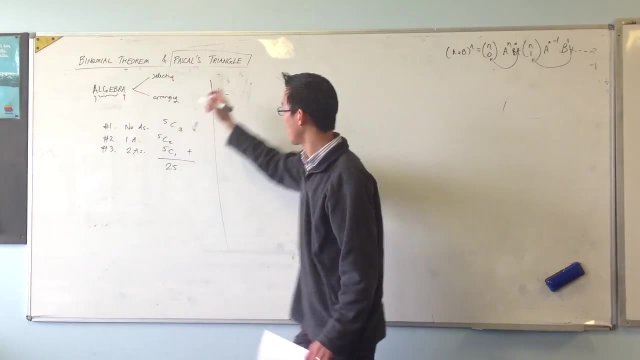 So I think the first way I thought about it was: forget about the fact that I've got to double up A, So I've got A, L, G, E, B and R Now. order matters now, So that's where I'm going to put together my box. 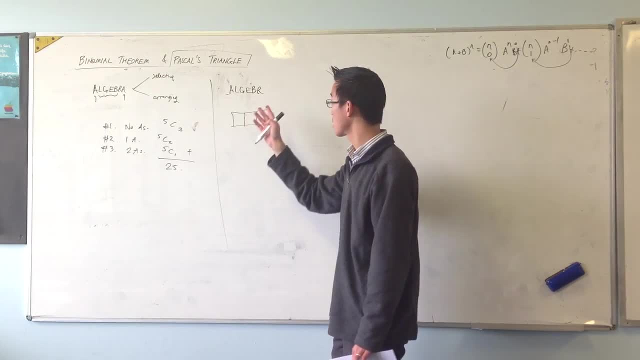 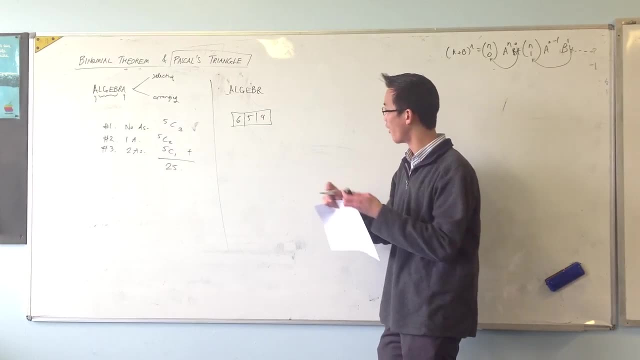 So in this scenario, here this is just 6P4.. Right, 6 by 5 by 4.. 6 factorial on 3.. Hold on, is that right? 3 factorial: Yeah, OK, So there's going to be one of your options. 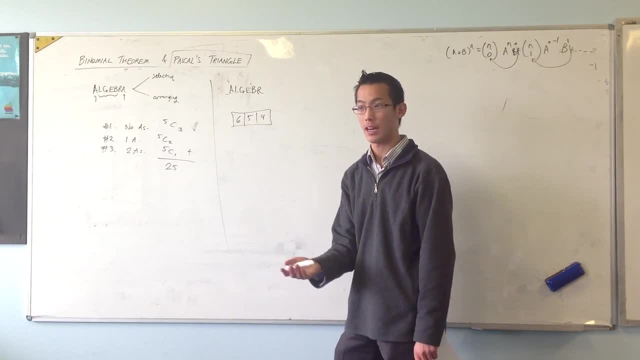 However, obviously I've eliminated the possibility here of having two, As which I can right. I can totally have that. Now, how many ways are there to have two As in there? I could have the two As bunched at the front. 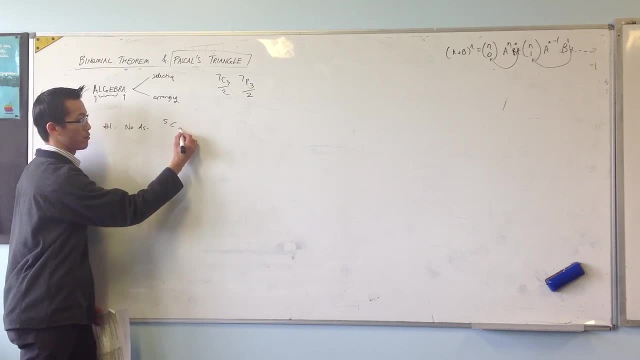 If I don't care about order. I've got five to choose from and I've got to choose three of them. Is that all right? Now, the second way is what if I have just one A? Now, don't forget, I don't care where the A is. 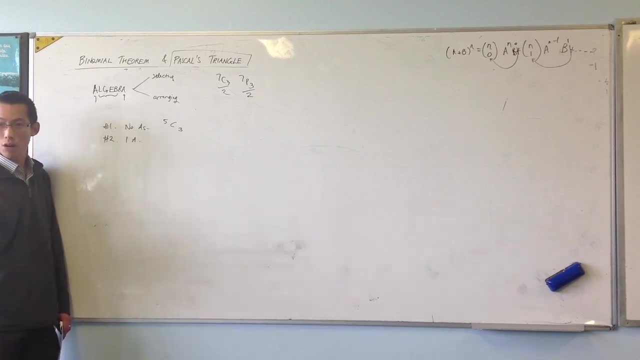 It could be at the start or the middle. at the end, If I've already chosen the A, I've got to make the other two letters from one of these five, And again I don't care what order. So I still have five to choose from, but I'm not choosing three. 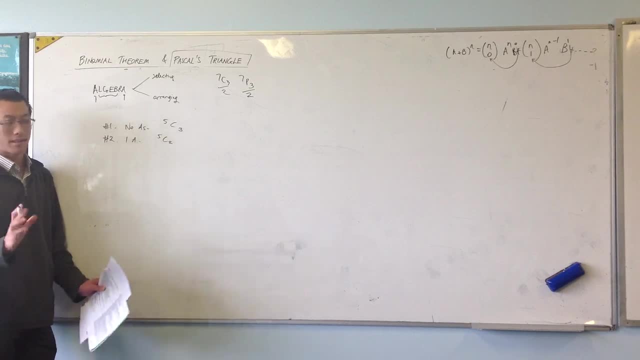 I'm choosing two. Last way. the third method is: what if I use both A's, So I could have them at the end, or I could have them bunched on the start or bunched at the end, But whichever way, remembering that I don't care about order, 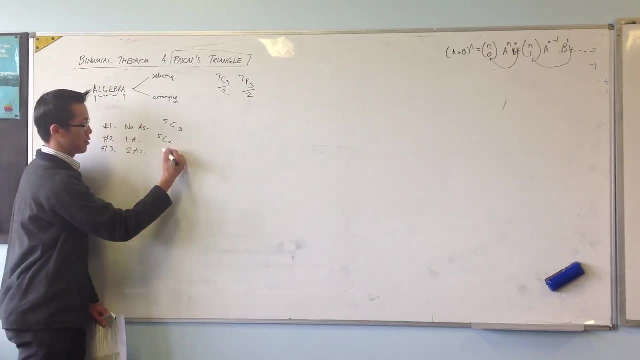 I have to pick one more letter to fill it out and I have to choose from five. So it's five, choose one. So when you add all of them up, I think you get 25.. This would be five, This is ten, and this is ten as well. 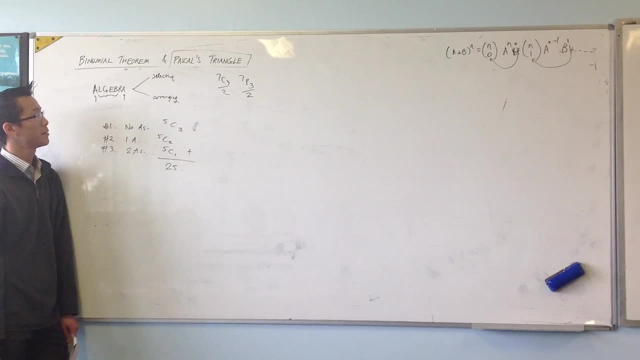 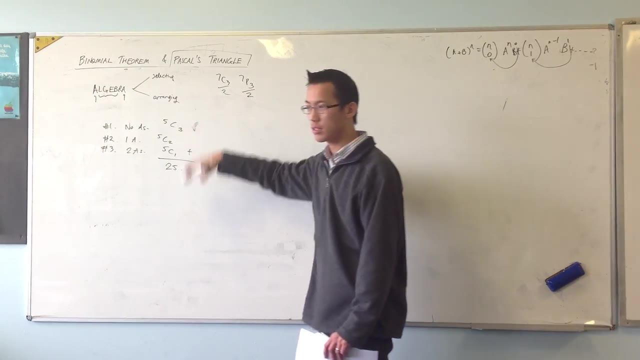 I think that's the way it works. So there's your 25,, which is the answer. How, then, do you go about it when you think about when order matters? You've still got to do a similar thing here. Let me make sure I read this properly. 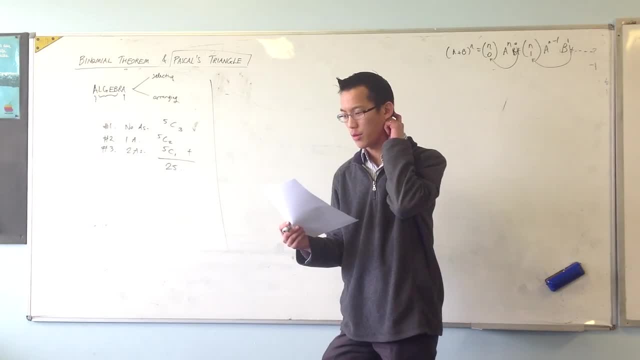 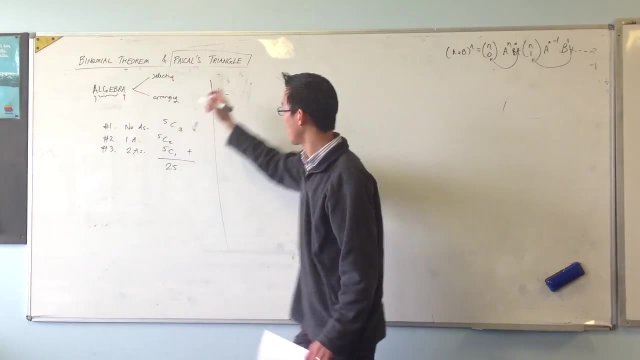 So I think the first way I thought about it was: forget about the fact that I've got to double up A, So I've got A, L, G, E, B and R Now. order matters now, So that's where I'm going to put together my box. 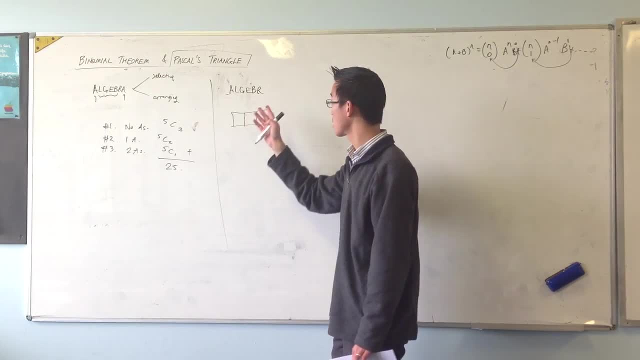 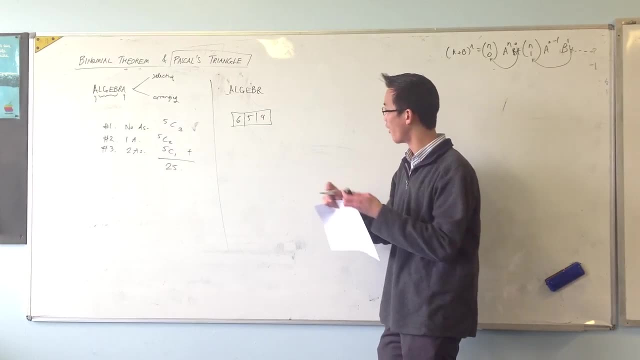 So in this scenario, here this is just 6P4.. Right, 6 by 5 by 4.. 6 factorial on 3.. Hold on, is that right? 3 factorial: Yeah, OK, So there's going to be one of your options. 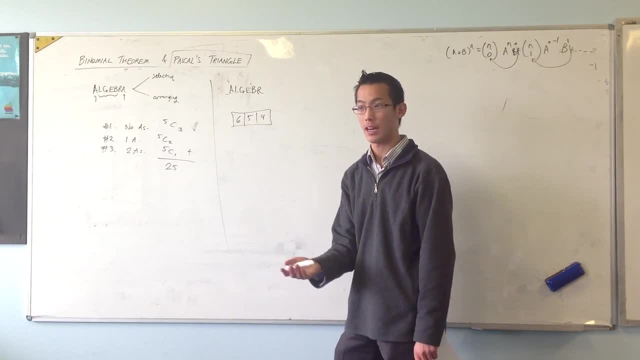 However, obviously I've eliminated the possibility here of having two, As which I can right. I can totally have that. Now, how many ways are there to have two As in there? I could have the two As bunched at the front.